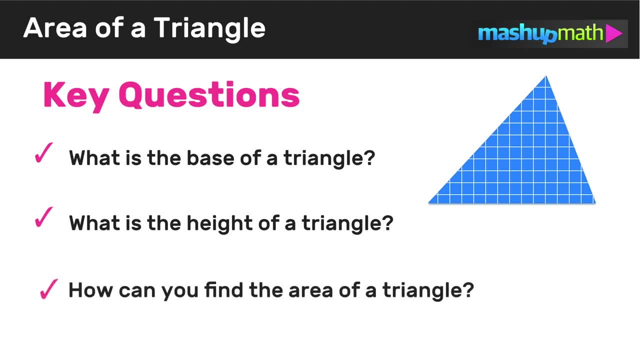 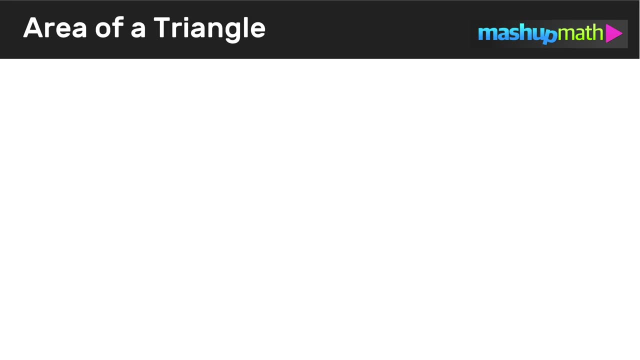 triangle. we have to explore what is the base of a triangle, what is the height of a triangle and how can you find the area of a triangle? So let's go ahead and explore those questions now. So let's go ahead and review some important triangle properties For 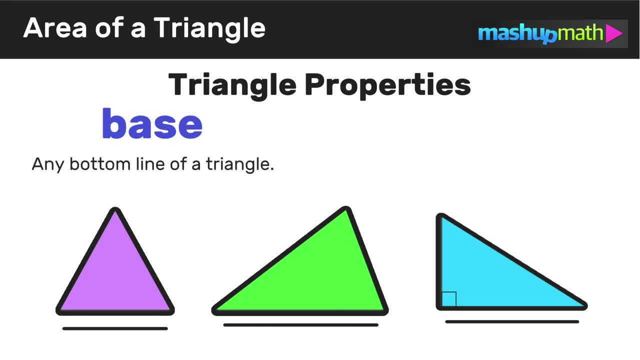 starters, the base of a triangle is any bottom line of a triangle, And we label the base of a triangle with the letter B, and B represents whatever value the length of that triangle base is. Now the height of any triangle is a perpendicular line that extends from the base of a triangle to the vertex of the. 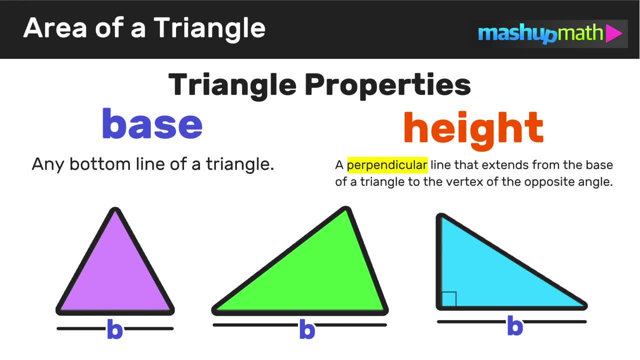 opposite angle. So let's take a look at what that means and what that looks like. So the height of a triangle is a perpendicular line, that's a line that runs from the base, forming a right angle with the base, and it extends all the way. 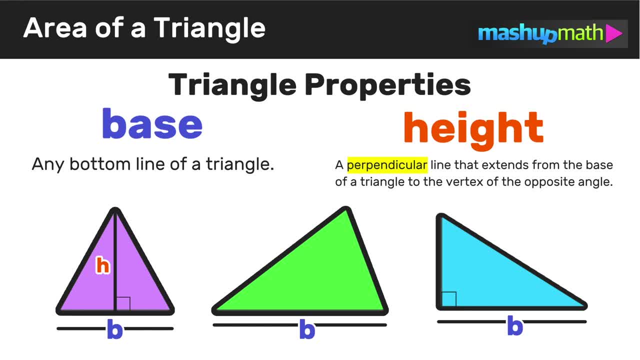 to the, the opposite angle, the angle directly across from the base, and we are going to label the height of a triangle with the letter h, and again, h represents the value of that height, the length of that line. and just a quick note on finding the height of a right triangle, since a right triangle already has. 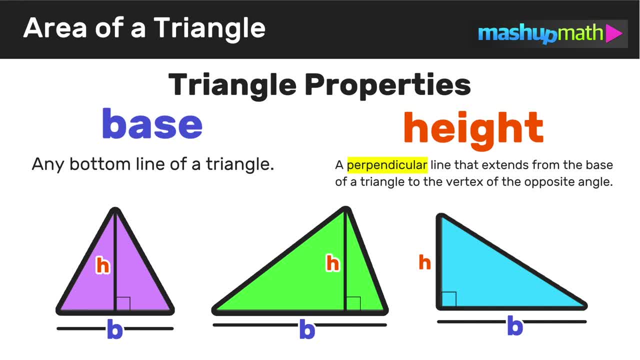 a pair of perpendicular lines, the height will be the side directly adjacent to the base. so the side adjacent to the base. that's not the hypotenuse. so as long as you can identify the base and height of a triangle, you can find the area of that triangle. so now let's go ahead and learn exactly. 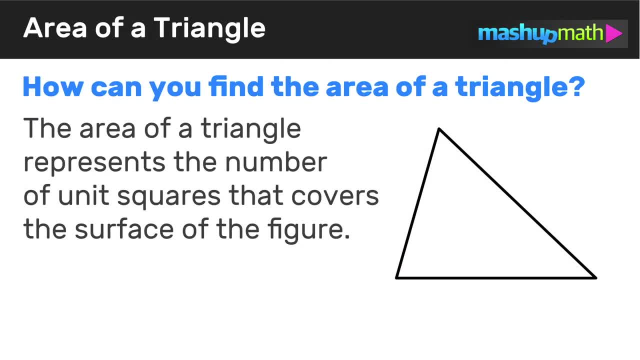 how to do that. so how can you find the area of a triangle? so we are going to say that the area of a triangle represents the number of unit squares that covers the surface of the figure. so let's now visualize what that means you. so when we say unit squares, we're saying how many unit squares it will take to cover the surface. 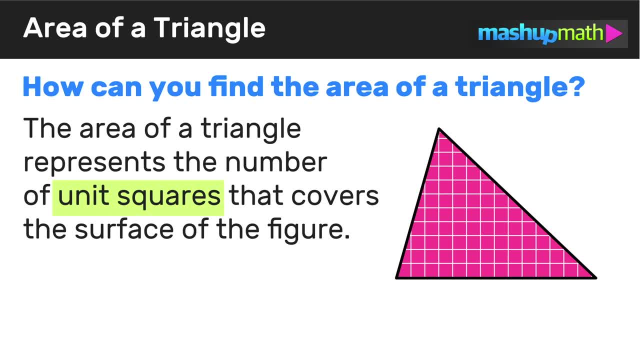 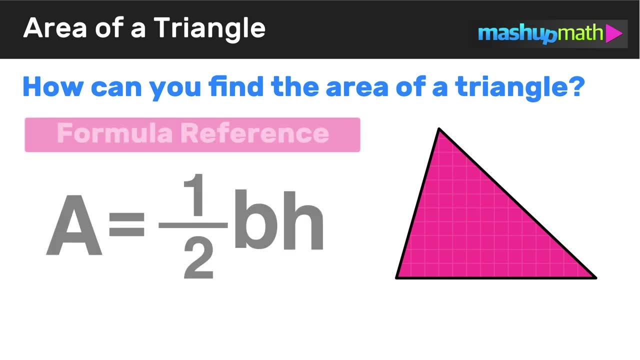 of the triangle and our unit square depends on what unit we're working with, whether it be square centimeters or square inches or square meters. area is always expressed in square units and to find the area of a triangle we are going to use a formula, and the area of a triangle formula is a equals one half times the base, times the height, so as: 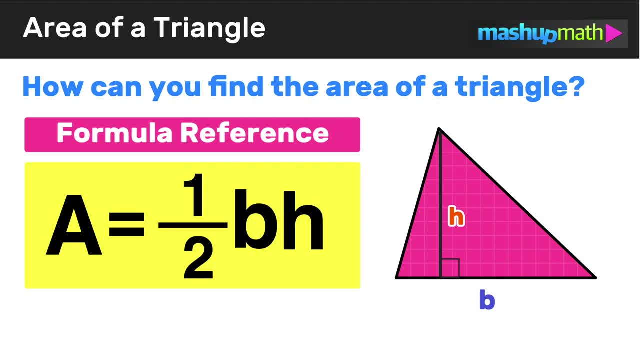 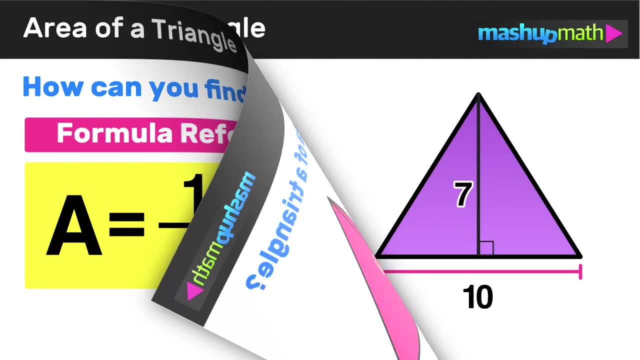 long as you know the value of the base and the height of a triangle, you can plug those into the area formula and you can figure out how many unit squares make up the area of the triangle. so now let's go ahead and look at a few examples of how to use the formula. all right, so now we're ready for. 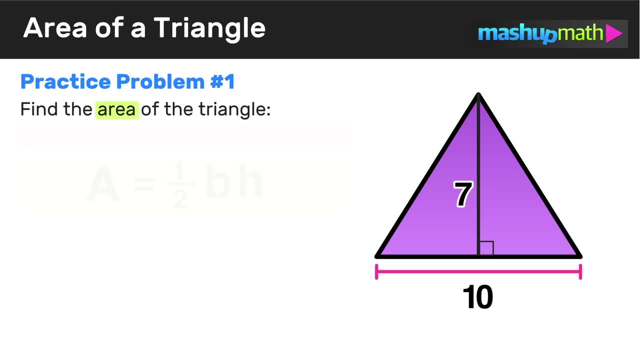 for our first practice problem, and in this problem we have to find the area of the triangle shown. So we should know that to solve this problem we have to use the triangle area formula. Again, the formula says that a equals one half base times height. Now let's take a look at that. 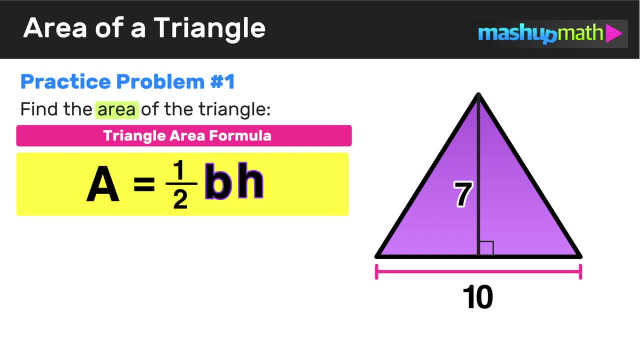 diagram and identify the base and the height. If we know those two values, we can just plug them in, So we can see that the base of the given triangle is equal to 10, so we know that b equals 10, and we can see that the height of the given triangle is 7, so we know that h is equal to 7.. 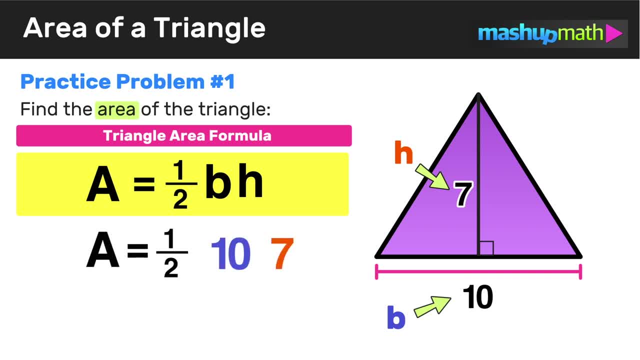 So now let's go ahead and rewrite the formula, replacing b with 10 and h with 7.. So now, instead of area equals one half times b times h, we have area equals one half times 10.. Again, because in this triangle b equals 10 and h equals 7, so we just substituted those values in. 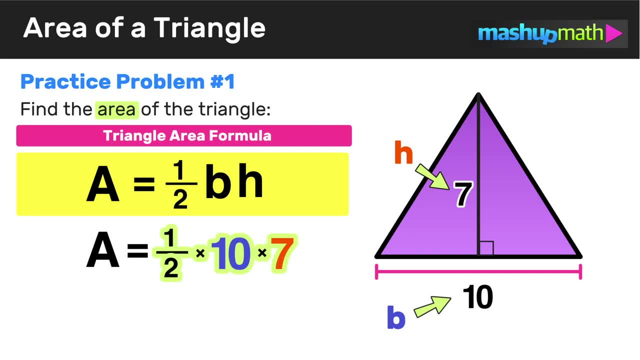 and now we can go ahead and multiply and we can figure out the area, And so one half times 10 times 7 is equal to 35, and remember that area is measured in square units. So the area of this triangle is 35 square units and that's all there is to it. 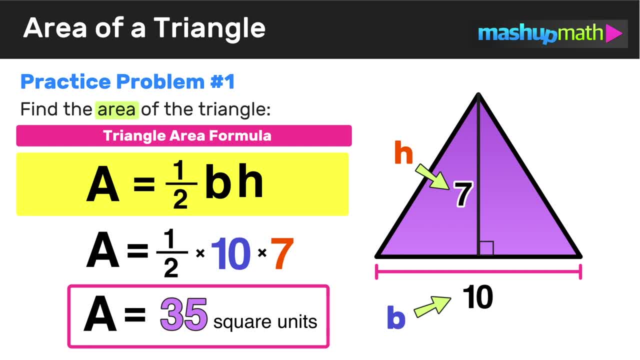 So that's exactly how you use the area of a triangle formula to solve a problem. but if you're still learning this and this is new to you and you're trying to get the hang of it, let's go ahead and look at another practice problem. 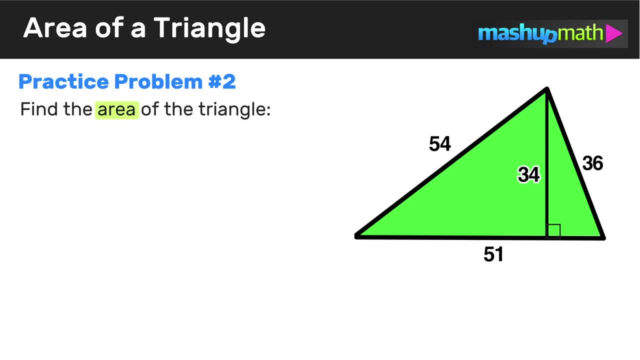 Okay, so here's practice problem number two, and just like the last example, we have to find the area of the triangle, and we're going to use the triangle area- formula a equals one half times b times h- to figure that out. So let's go ahead and figure out the values of b and h for this triangle. 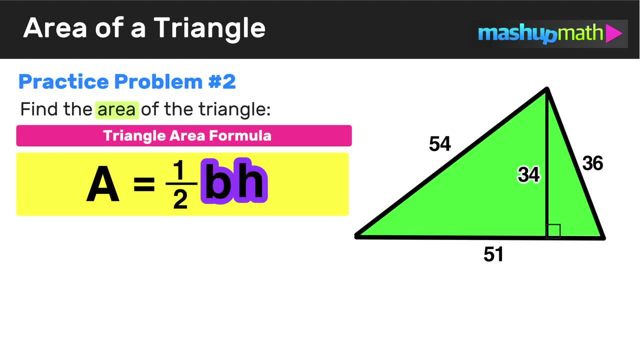 Now, the last example had less information giving on the diagram. This one has more sides labeled, but remember, the base is any bottom line of the triangle. So the base of this triangle is 51 and the height is that perpendicular line that extends from the base. 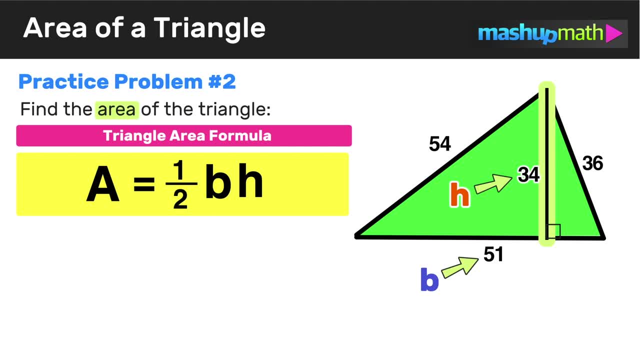 to the vertex of the opposite angle. So in this example the height is 34.. And remember to use the area of a triangle formula. all we need is the base and height, So we don't have to use those two other sides of the triangle that are already labeled. 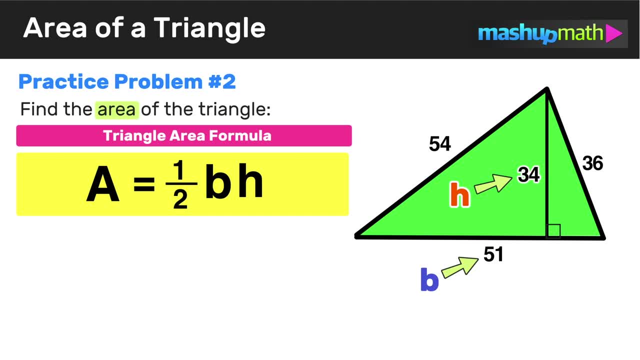 the 54 and the 36.. We don't have to use those at all. Okay, so since we know the value of b and the value of h, we can go ahead and plug them into the area formula. So now we have: area equals one half times 51 times 34.. 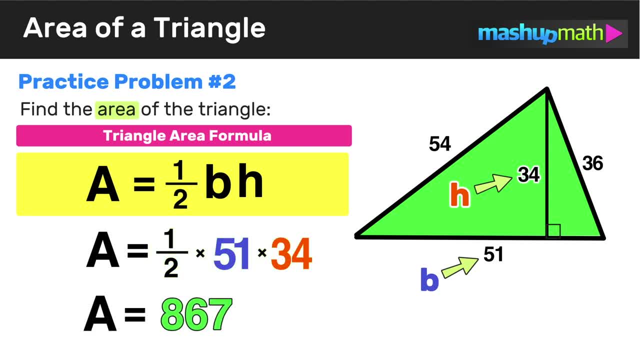 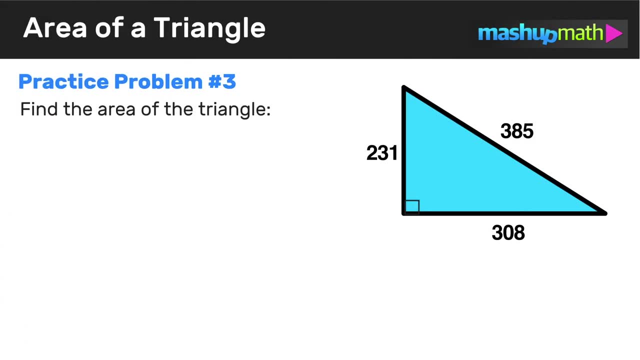 And that product is equal to 867.. So we can conclude that the area of this triangle is 867 square units. And now we are ready to take on the third and final practice problem, And again we have to find the area of the triangle given. 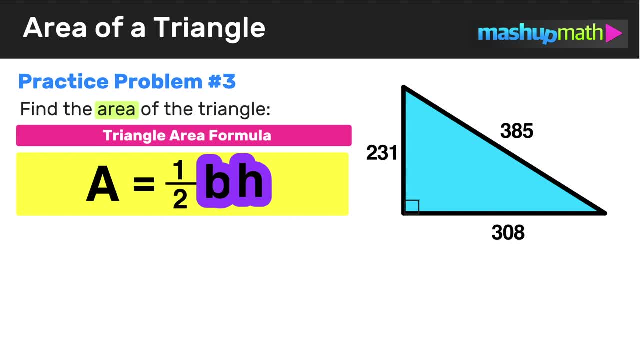 and we're going to use the triangle area formula To do that. so let's go ahead and identify the values of b and h, the base and height of the right triangle in this example. So, looking at the diagram, we can see that the base of this right triangle is 308.. 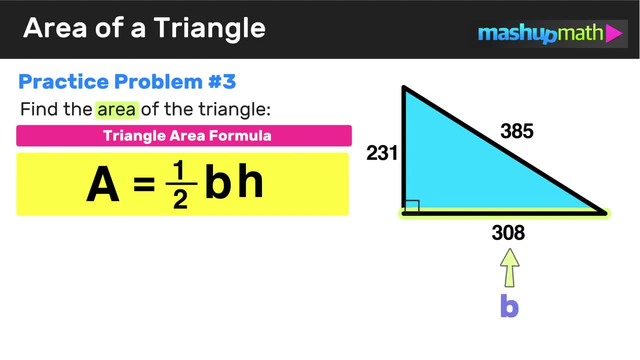 So we can label the base with the letter b and in the formula we can replace b with 308.. And since this is a right triangle, we know that the height is the perpendicular line from the base that is adjacent to the base, And in this case it's 230..